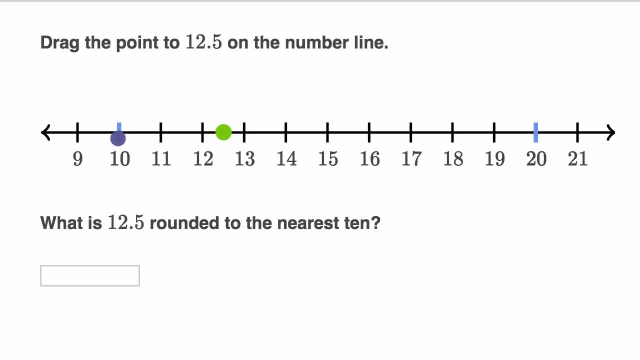 Which is literally the nearest 10?? Well, you can see we are closer to 10 than we are to 20.. So you would say 10.. And this helps us build an intuition for what rounding to the nearest 10 even means. 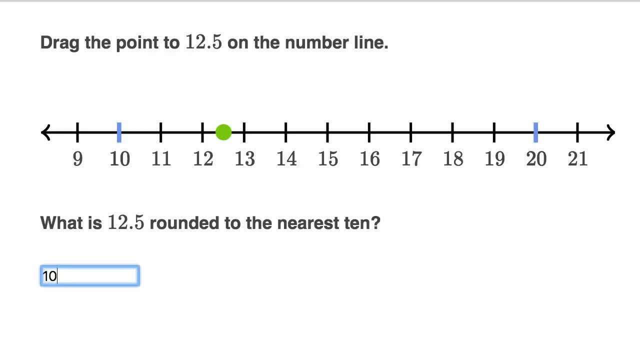 Because you might know a rule like: hey look, you go one place less than the 10s place, which would be the ones place, And if it's less than five there, you round down to 10.. If it's five or greater, you round up to 20.. 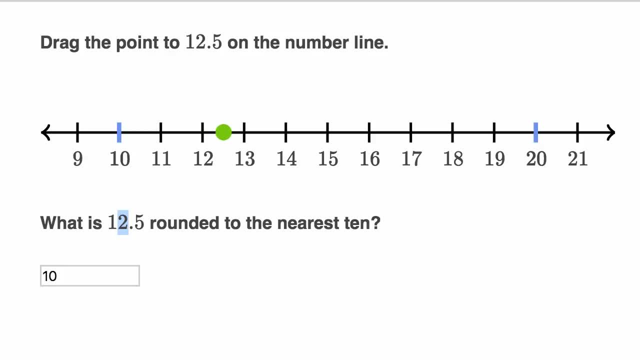 But do you see why? over here We are just closer to 10.. Let's do another example here. So here it says: drag the point to 0.136.. So this is 0.13,, this is 0.14.. 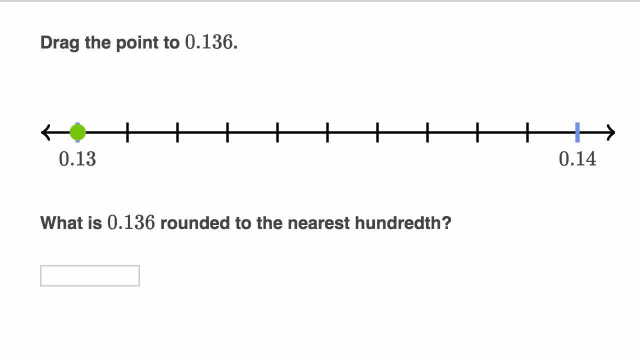 So this is 13 hundredths, and this is 14 hundredths. And let's see, there's one, two, three, four, five, six, seven, eight, nine, 10.. So these are, you could think of it as the 10 thousandths. 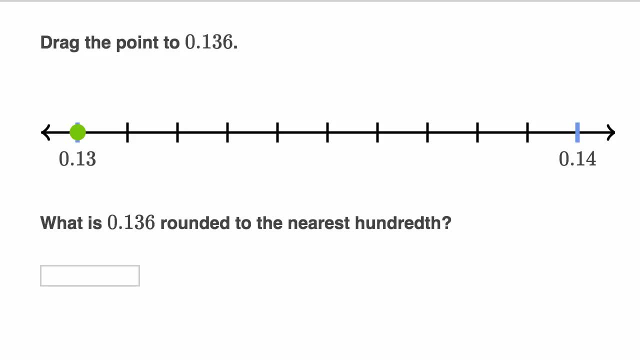 between these two hundredths. So we wanna go 13 hundredths and then another six thousandths. So let's see, we go one, two, three, four, five, six, just like that. And then they say: what is this number? 136 thousandths. 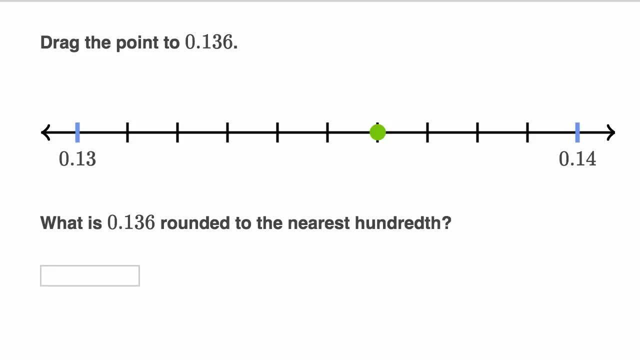 or 0.136, rounded to the nearest hundredth. Well, we have our hundredths in blue here. and which one are we closer to? Well, we're closer to 14 hundredths: 0.14.. And that's consistent with what we've seen in other cases. 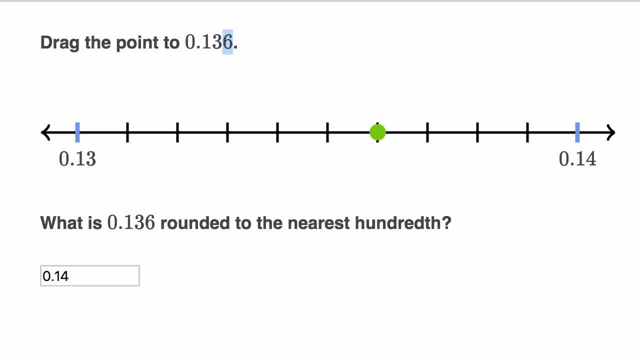 where you look at the thousandths place and if it's five or greater, you round up. In this case, you would round up to 14 hundredths. Let's do a few more. Let's look at some more examples here. 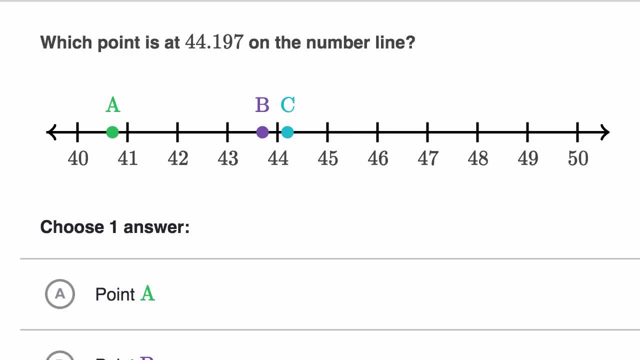 So let's say that. so they're asking us which point is at 44.197 on the number line. So let's see that's going to be between 44 and 45, so it's right over here 44.197,. so that would be point C. 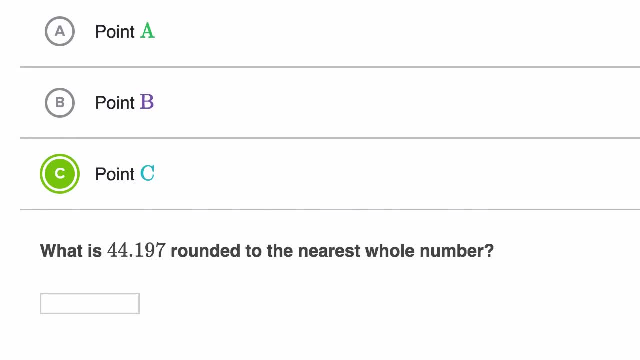 And then they say: what is? 44.197 rounded to the nearest whole number? Well, there's a couple of ways to think about it. So let's look at the hundredths place and say, look, that's less than five. so we round down to 44..